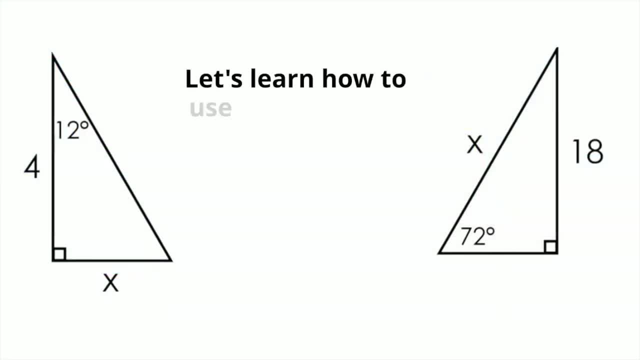 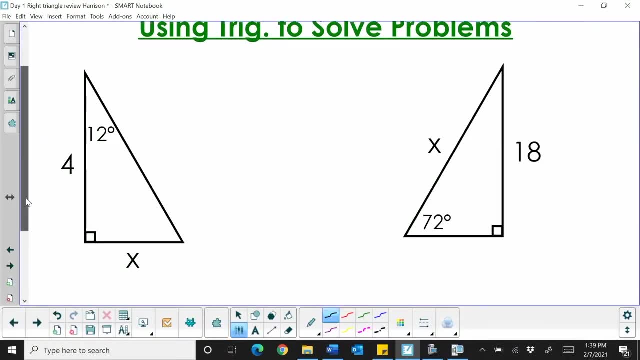 Okay. so let's try a couple of these where we have to figure out which trig function. So, using trig solve these problems, And we're just solving for one variable. So if this angle is 12, this side is 4, which trig function would I use to find the missing side? 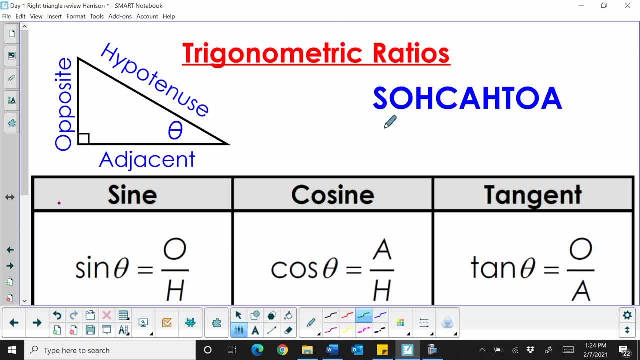 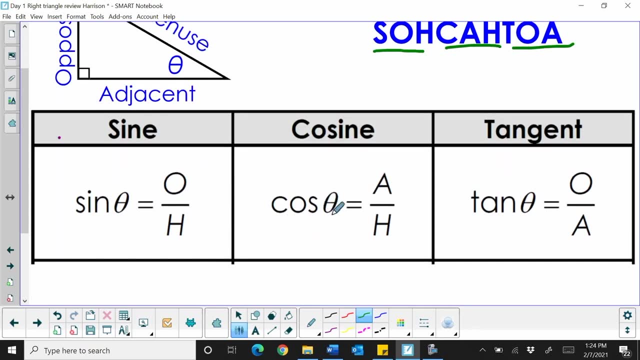 And review trig ratios. So our trig ratios are sine, cosine and tangent, where sine is your opposite over hypotenuse, Cosine of an angle is adjacent over hypotenuse And tangent of theta is equal to opposite over adjacent. And a lot of you learned just so. 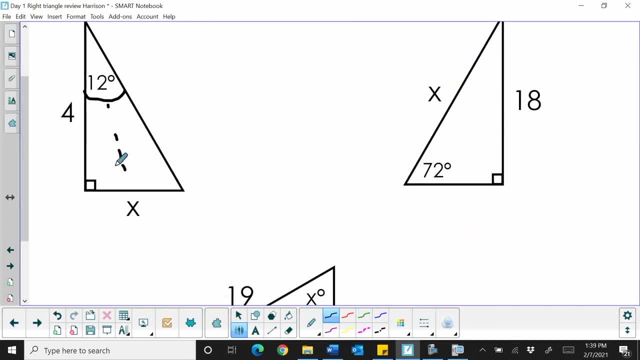 katoa to help Remember that. Well, let's identify This. one is opposite, This is another leg, so it's adjacent. which trig function uses opposite adjacent and that is tangent. So tangent of the angle, which is 12, is equal to x over 4.. Grab your handy dandy calculator and take the tangent of. 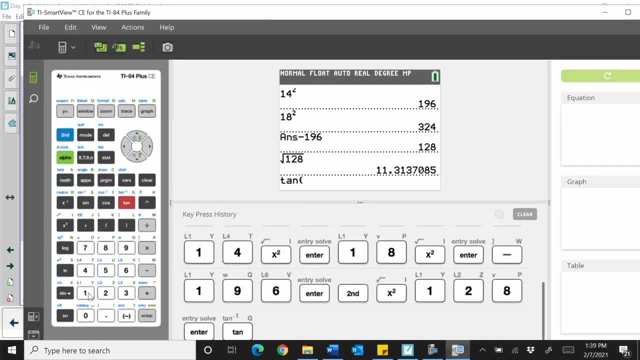 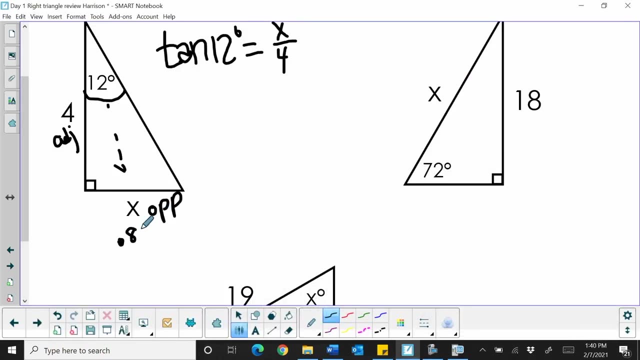 12. Close that bracket. If not, you're going to multiply the angle times 4. And that's going to give us 0.85.. So that means this side over here is 0.85, which is less than 1.. Well, let's see if. 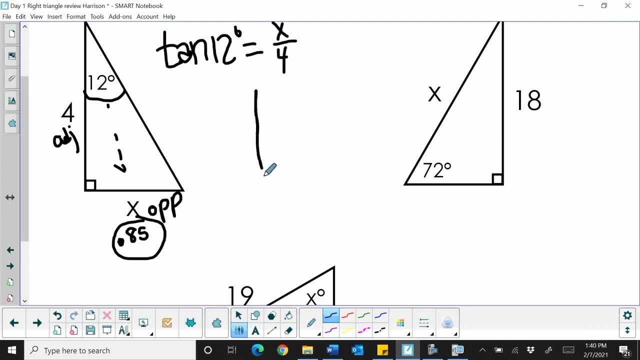 that makes sense. If this angle is only 12,. if we were to draw that to scale, it would look something like this: Very small, Where this is 4, and that's not even 1.. Yes, that does make sense. It's going to be less than 1.. So 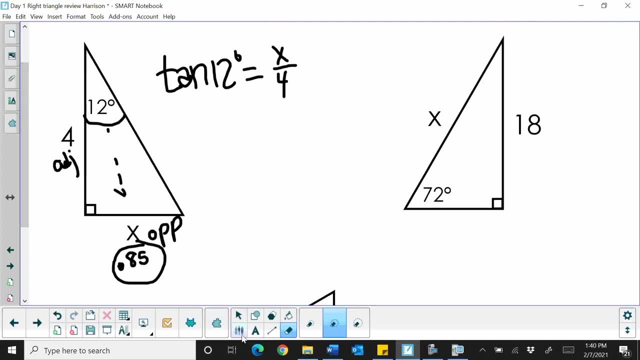 think about that kind of logically. Okay, let's look at the second one. Okay, we have an angle that's 72. This side is our opposite. We're trying to solve for the hypotenuse Which trig function do you use Opposite hypotenuse, that is sine. So the sine of 72. And we're going to